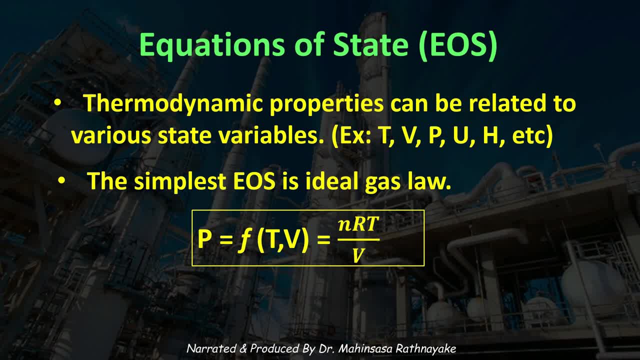 Even for energy constant為se through electrone rubber, We could proceed to the next risk. eleven with be done or by going to the next step. This is the world's study of thermodynamics interactions For non-ideal systems. equations of states should be developed. 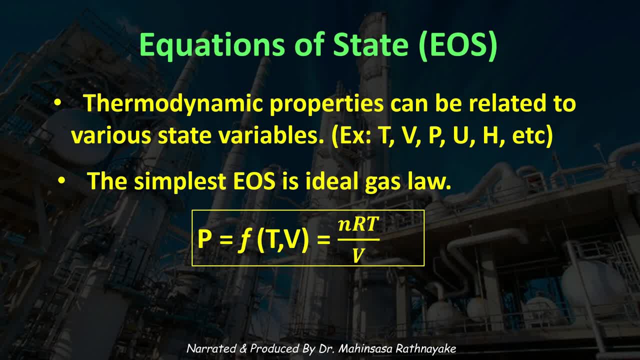 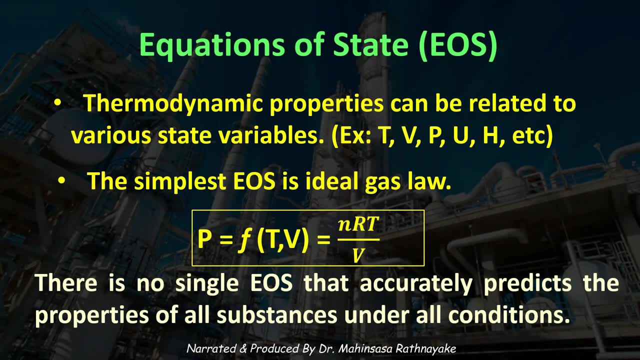 with more parameters, as their properties can vary with different conditions. Keep in mind that there is no single equation of state that accurately predicts the properties of all the substances under all conditions, So we should select the most appropriate equation of state for our applications during simulations. to 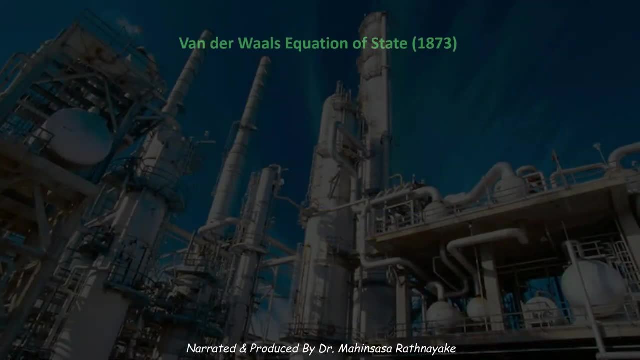 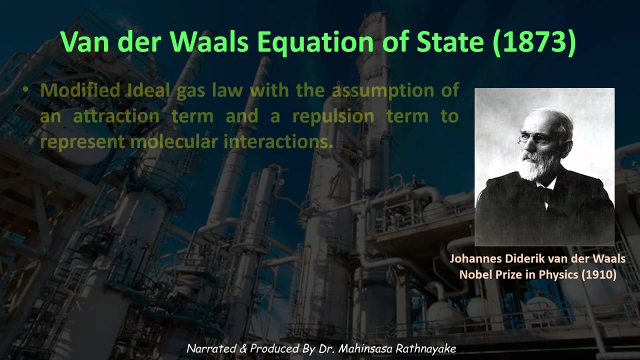 obtain more accurate results. Van der Waals equation of state in 1873 can be considered as the first equation of state in the world. Hope that you have heard of Van der Waals, who discovered liquid helium and won the Nobel Prize in physics in year 1910.. Van der Waals. 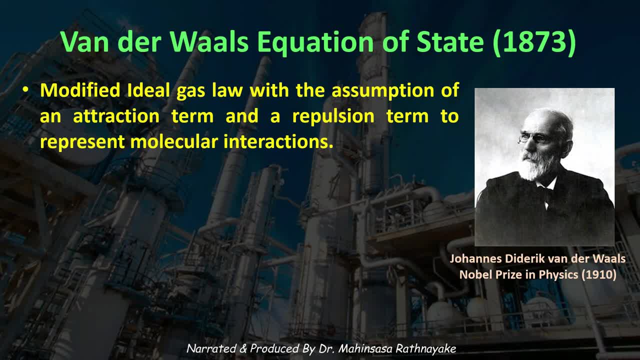 proposed an equation of state by modifying the ideal gas law with the assumption of an attraction term and a repulsion term to represent the molecular interactions. You can see the Van der Waals equation of state on the screen now, The negative term of a square of molar. 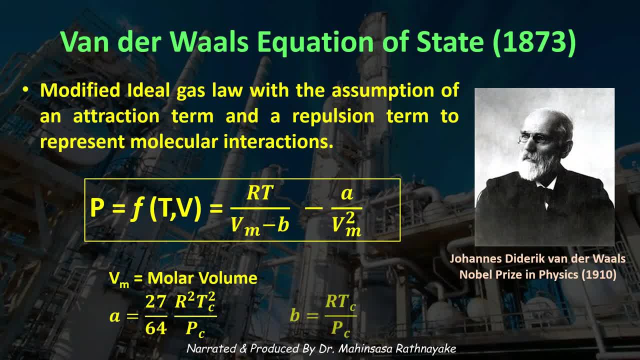 volume is the attraction term. The molar volume minus b is the repulsion term. Furthermore, the parameters a and b are the functions of critical properties. However, there are modern equations which are much more accurate than Van der Waals equation of state. 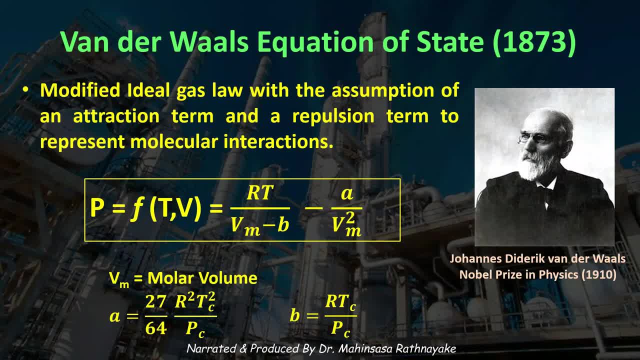 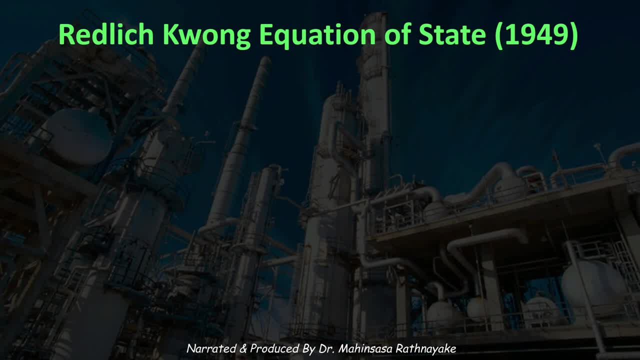 State Introduced in 1949, the Redlich-Quan equation of a state is such a superior equation than Van der Waals, Even though it performs poorly with respect to the liquid phase. it can be used in conjunction with separate liquid phase correlations to accurately calculate vapor. 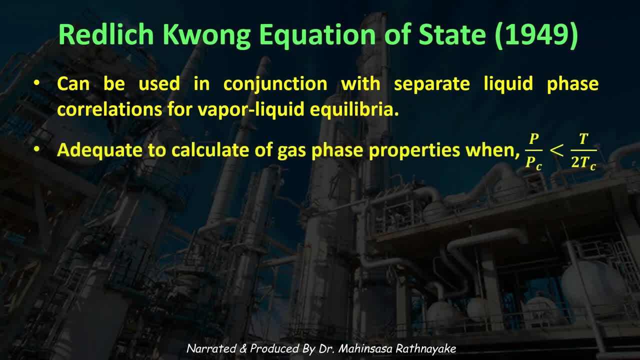 liquid equilibria. However, the Redlich-Quan equation is adequate for calculation of gas phase properties when the ratio of the pressure to the critical pressure is less than about half of the ratio of the temperature to the critical temperature. You can see the Redlich-Quan equation. 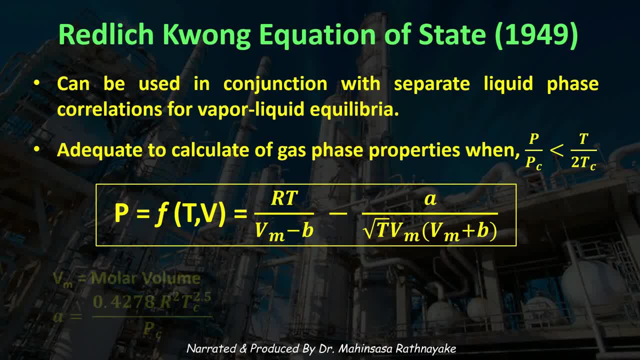 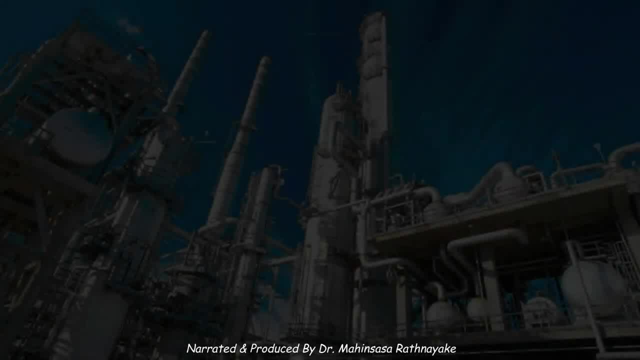 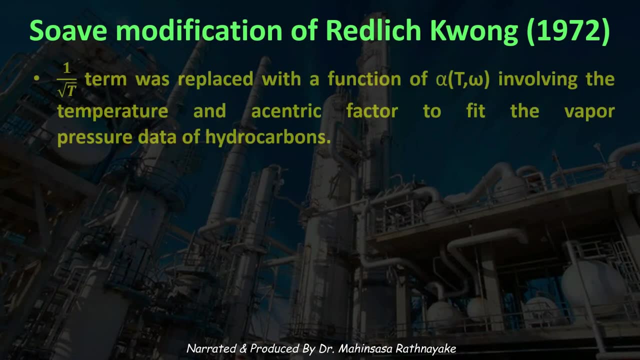 of a state on the screen. It has a more complex attraction term than Van der Waals. In 1970, the Redlich-Quan equation of a state was used to calculate the pressure of a gas phase. In 1972, the 1 over square root t term of Redlich-Quan equation was replaced by so with the function of. 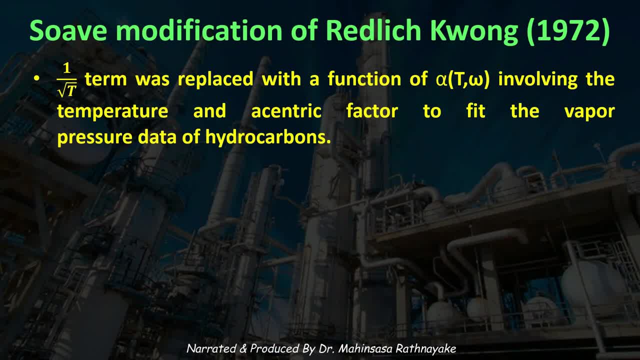 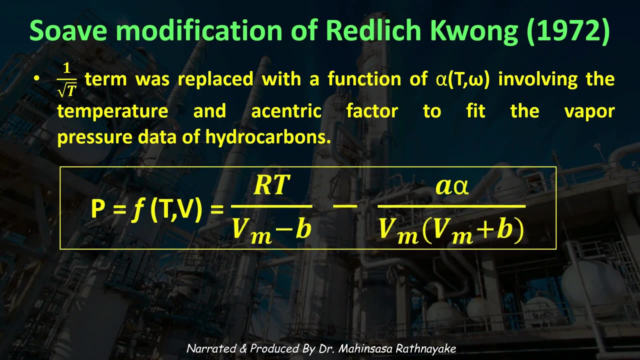 alpha involving the temperature and the eccentric factor to fit the vapor pressure data of hydrocarbons. The equation fairly fits for the data and the resulting equation is known as the Soh-Redlich-Quan equation of a state. You can see the Soh-Redlich-Quan equation of a state on the. 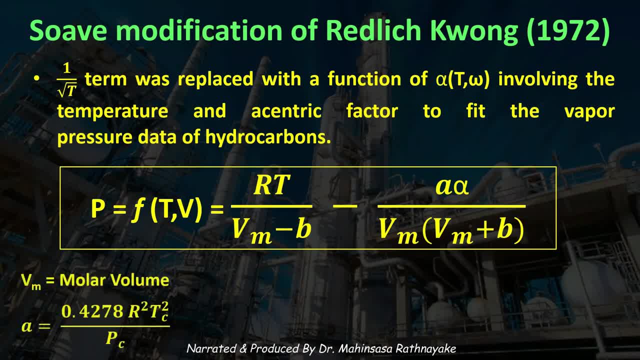 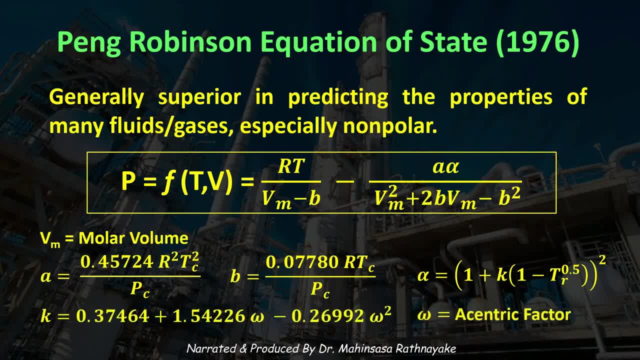 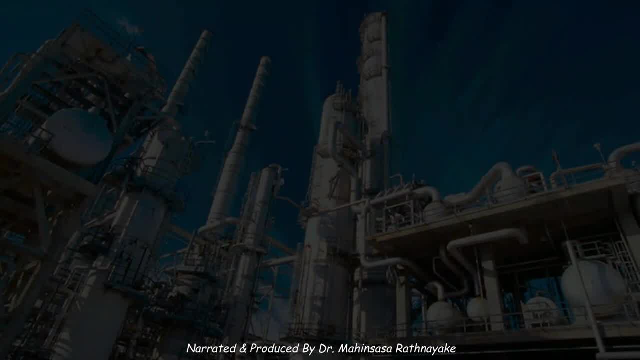 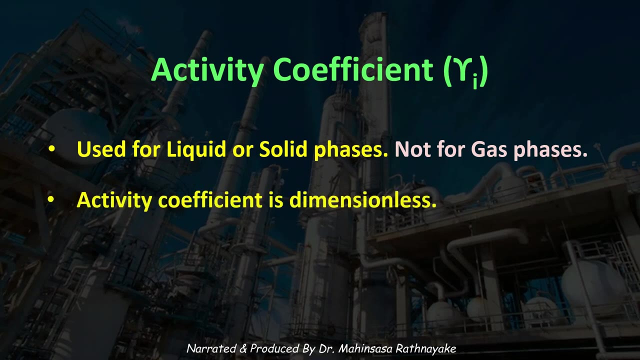 Note that after the replacement changes, the critical temperature is now in the second power. Next, let's briefly discuss what activity coefficient is. Keep in mind that activity coefficient is almost always used for liquid or solid phases and not for gas phases. It is dimensionless and noted by γi for a given component. 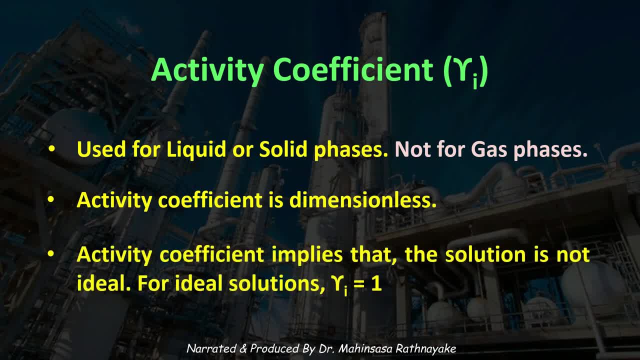 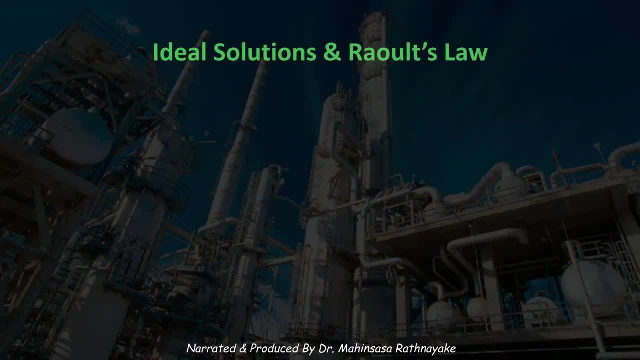 coefficient implies that the solution is not ideal. For an ideal solution it is equal to 1.. For example, if we have A and B that are mixed together, then the interactions between A molecules and B molecules are the same as the interaction between A molecules and A molecules. Same that. 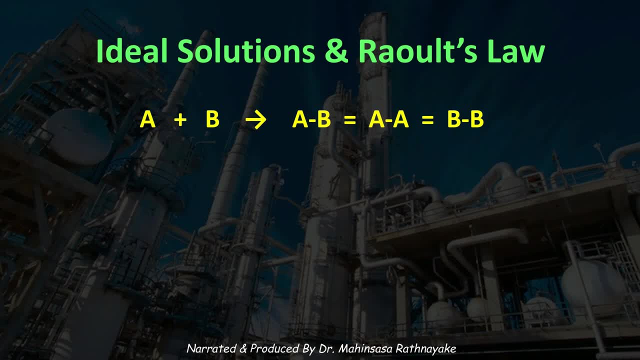 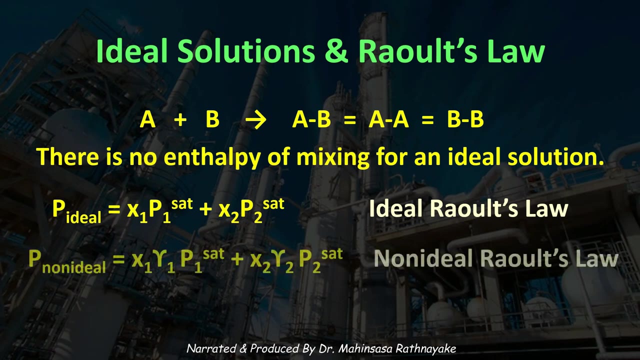 for interactions between B molecules and B molecules. In other words, there is no enthalpy of mixing. for an ideal solution, You can see the Raoult's law for an ideal binary solution on the screen. now For a non-ideal system, we add a correction factor gamma. So in the non-ideal 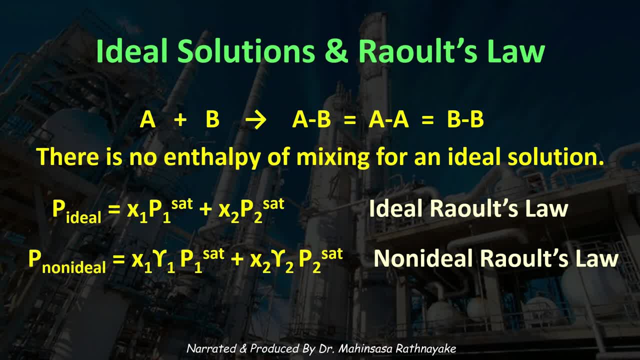 Raoult's law. there is a gamma term for each component, which indicates how much it deviates from an ideal system. If the pressure of the solution is greater than the pressure of the ideal solution, it is referred as a positive deviation from Raoult's law. This means gamma. 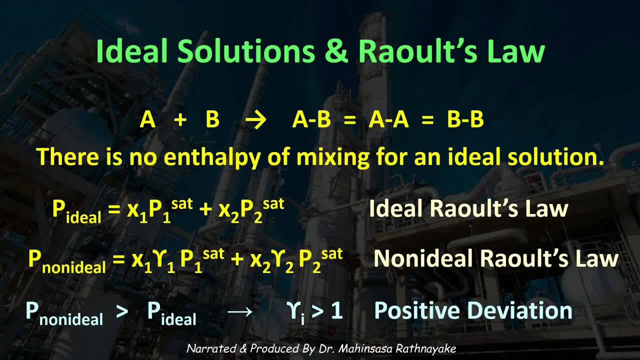 sub i is greater than the pressure of the ideal solution. Positive deviation means that the molecules don't want to be near each other. The pressure is higher because of their tendency to escape into the gas phase. Therefore the molecules have weaker interactions. The energy of bonding between A and B is less than between A and A or B. 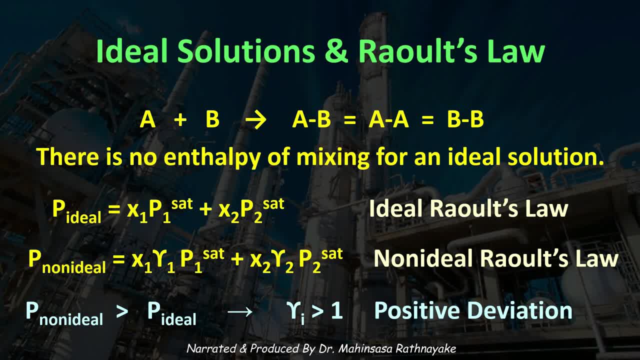 and B. now, More importantly, understanding of activity coefficient and related parameters is very beneficial in simulating phase equilibrium. for non-ideal solutions, In Aspen Plus software you can find many inbuilt property methods used in common component systems and unit operations. So if you feel difficult to understand the fundamental theories, 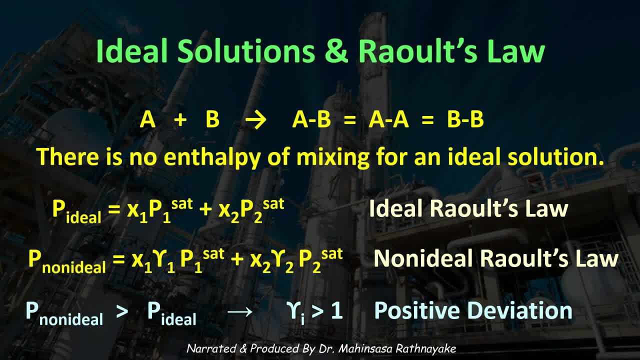 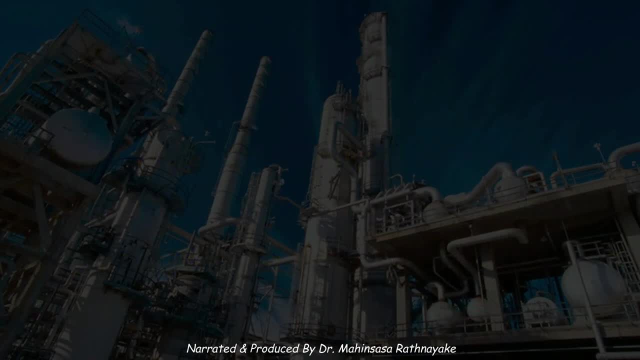 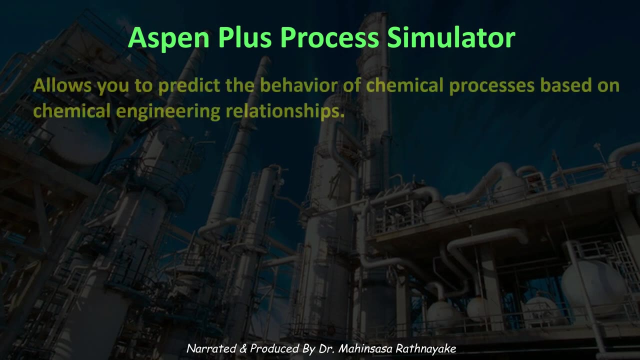 behind these property methods. at least try to know about what component systems or applications can be supported by each property method. Aspen Plus is a process simulator that allows you to predict the behavior of chemical processes based on chemical engineering relationships such as mass and energy balance phase and. 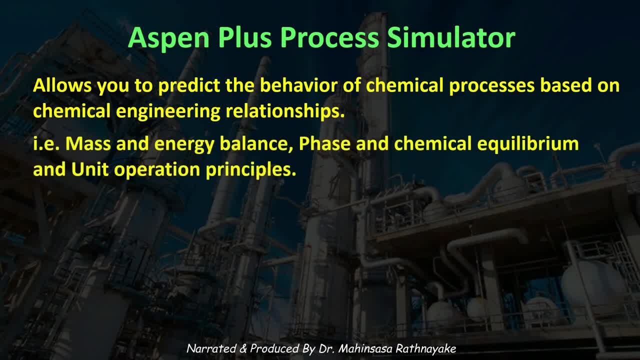 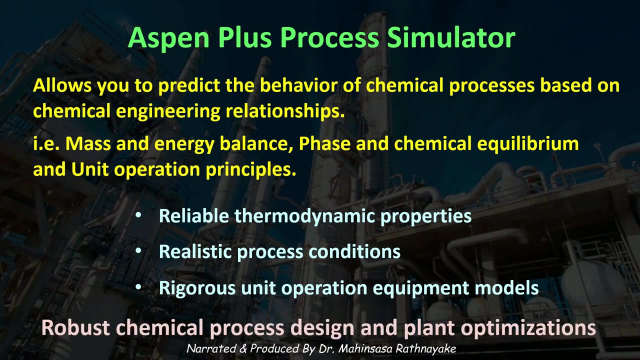 chemical equilibrium and unit operation principles. Given with reliable thermodynamic properties, realistic process conditions and rigorous unit operation equipment models, you can simulate actual process plant behaviors in a more robust manner. This saves a huge cost and time for chemical process design and plant optimizations. 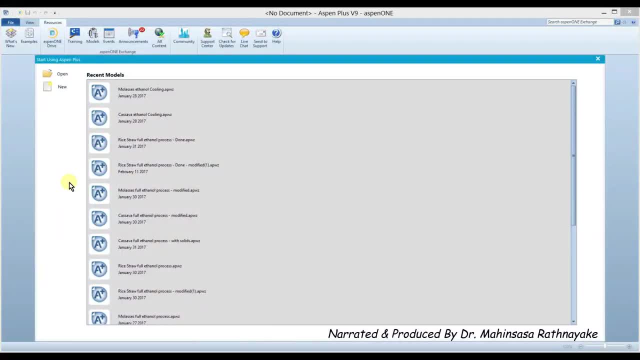 Let's open Aspen Plus software and get familiar with Help tab to learn more about available properties. You can click on the Help button in the menu bar to know about anything related to Aspen process simulations. Let's click the Help button and go to the Index tab. 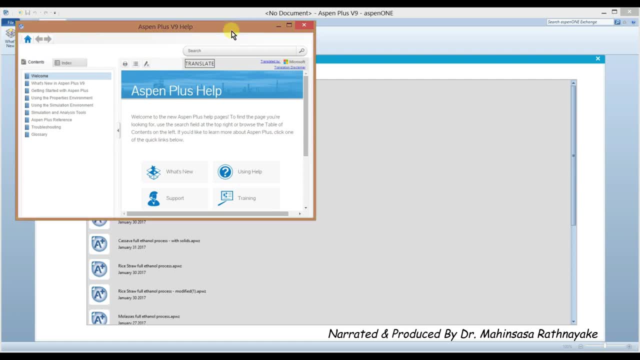 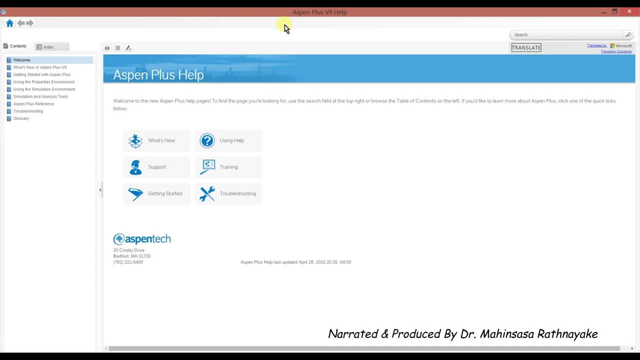 Aspen Plus is a process simulator that allows you to predict the behavior of chemical processes based on chemical engineering relationships, such as mass and energy balance. Aspen Plus is a process simulator that allows you to predict the behavior of chemical processes based on chemical operations. Let's click the Help button and go to the Index tab to learn more about available properties. 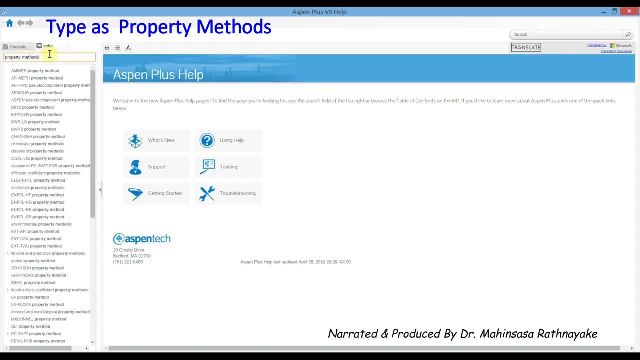 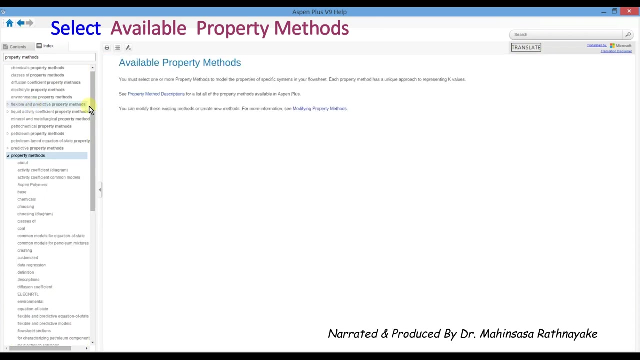 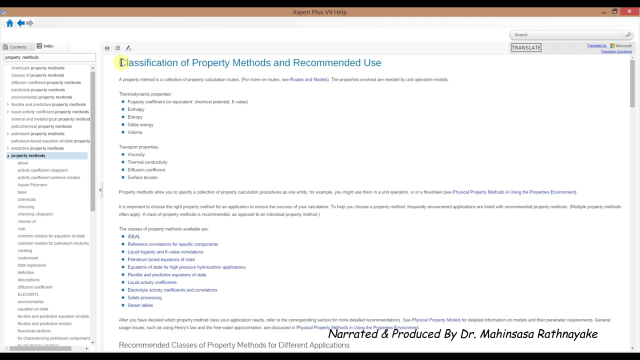 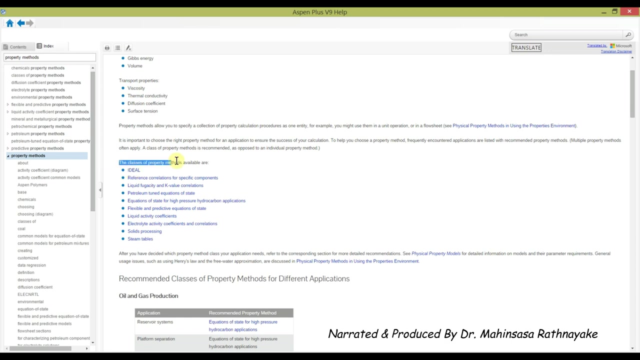 You can click the Help button and get familiar with Help % in the Index search bar. Aspen Plus has many functional functions and functions that allow you to measure a site Under the search, select Classification of Property Methods and Recommended Use option. Here you can see the different classes of property methods. 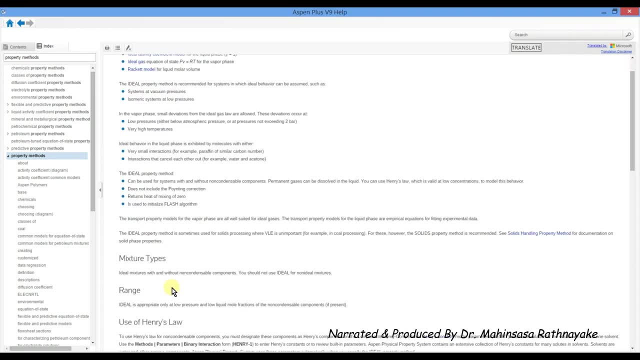 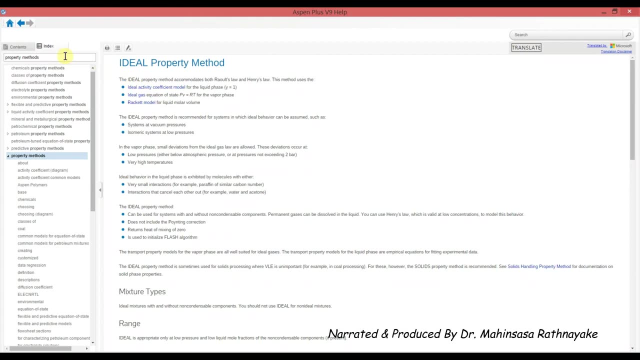 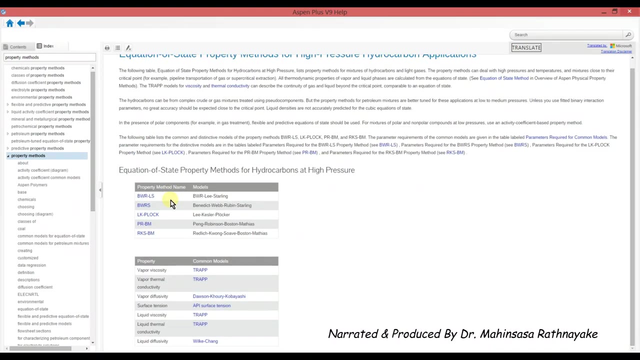 The ideal property method relies on ideal gas law, ideal Raoult's and Henry's laws to calculate the equilibrium distribution parameters of ideal systems. You can also see various equations of state property methods As discussed previously. the most popular are the Peng-Robinson and So-Redlich-Kwong. 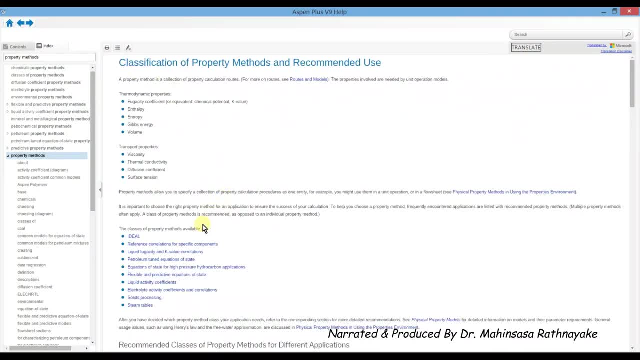 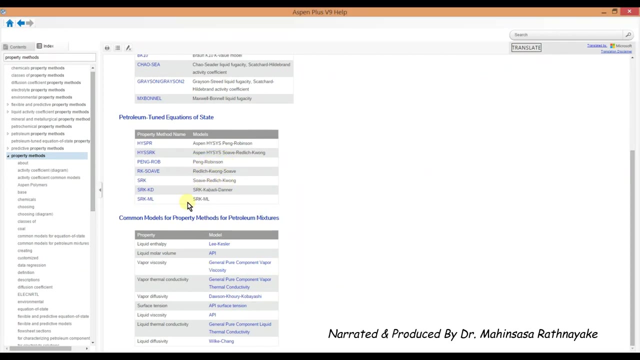 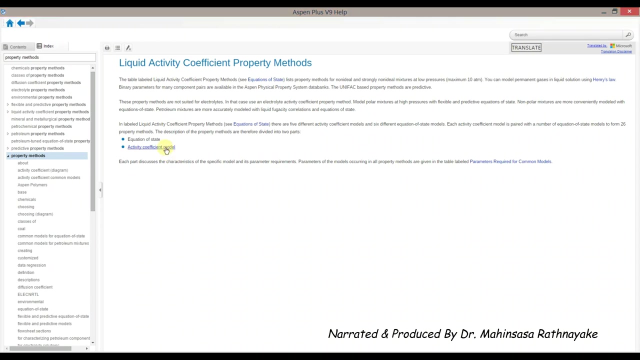 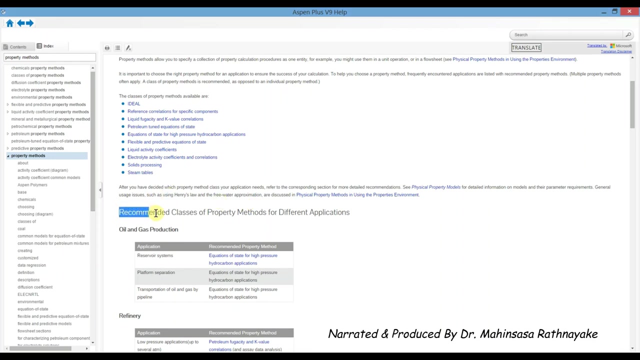 equations of state property methods. Next, you can learn about activity coefficient property methods that are used to calculate liquid phase activity coefficients And then evaluate the values. The widely used activity coefficient property methods are NRTL, abbreviated from non-random two-liquid, UNIFAC and Wilson property methods.